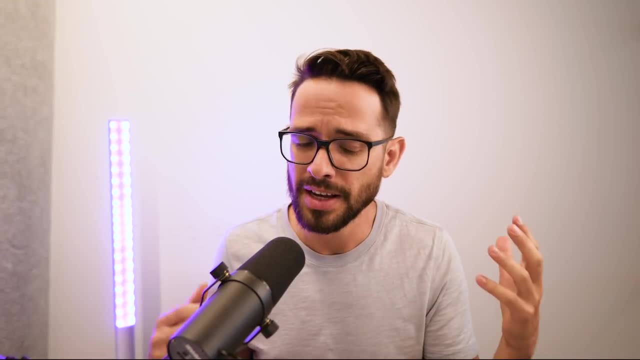 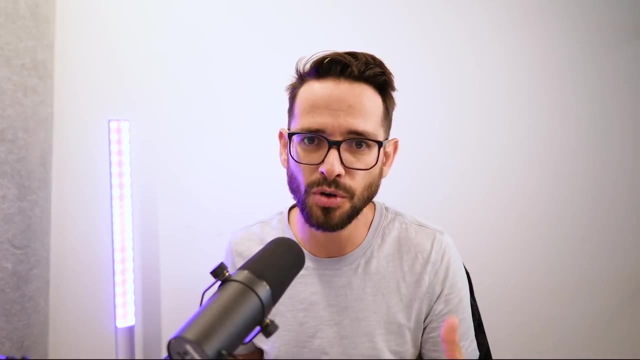 intro legislatively, like there was some new laws and there has been a rise in people who are actually suing website owners for not being accessible. So designers really need to understand what it is. So basically, let's cover what it is. The basic core concept is that not everybody has 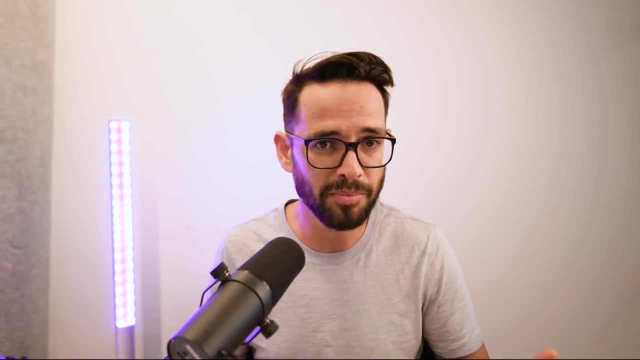 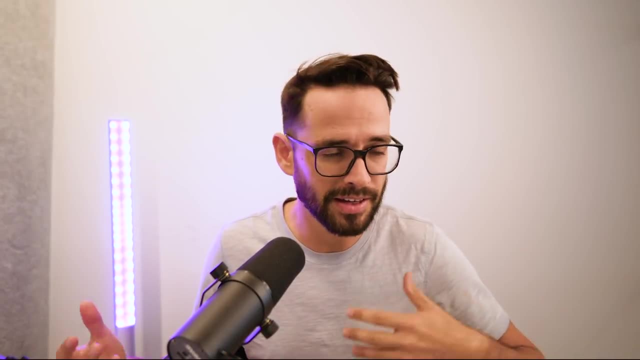 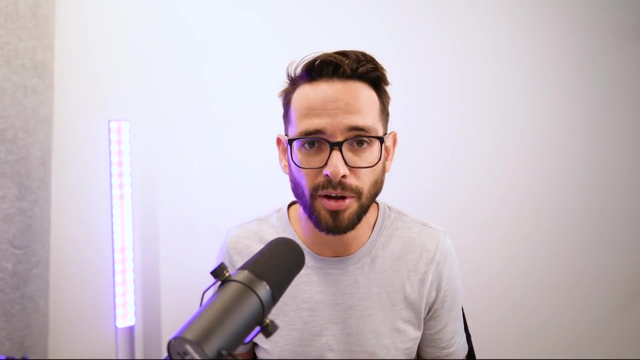 the same. you know, some people have disabilities. might be that they're not be able to see at all or have some kind of visual imparity, meaning they can't see color. well, they can't see, you know, as good as some other people. or maybe they can't, you know, they have some other. 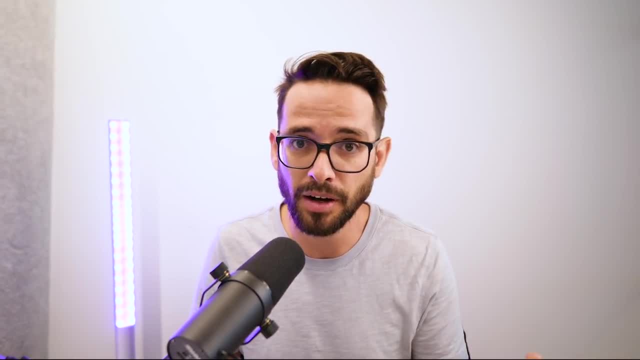 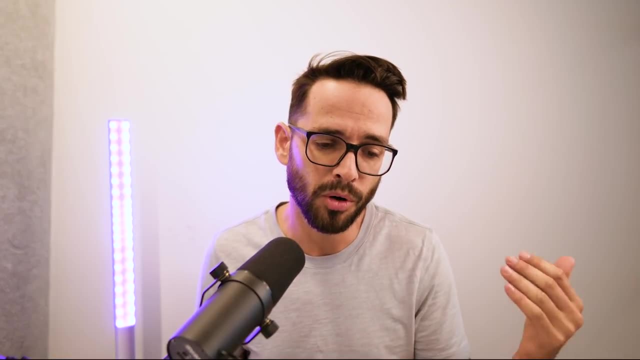 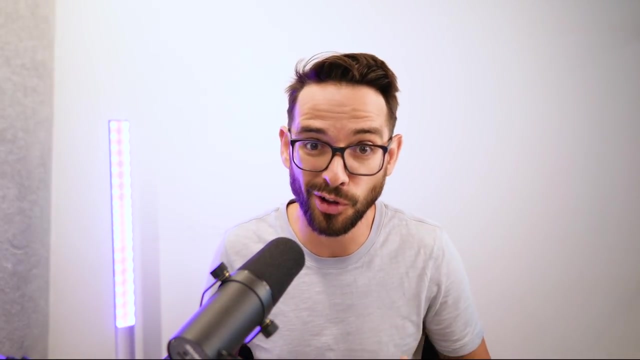 disabilities. So then maybe they're operating their computer and browsing through voice and through other tools, And so we need to make sure that those people will be able to browse the web as well. And it's kind of a basic right to be able to browse the web, And so we need to make sure that. 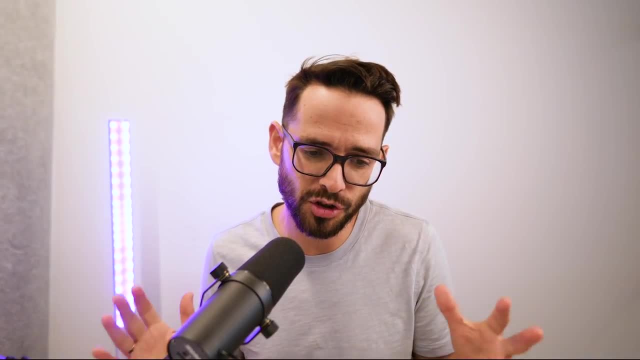 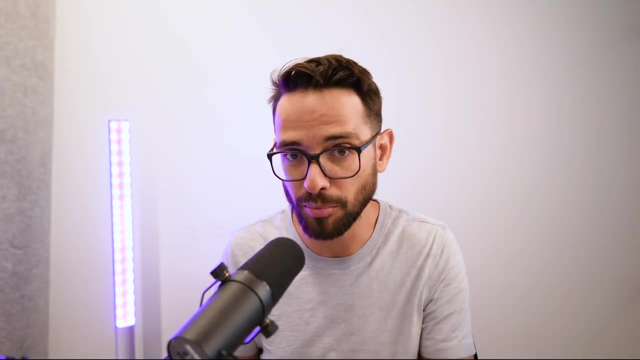 those people will be able to browse the web, And it's kind of a basic right to be able to browse the law these days. So there's basically two aspects to it. One of them is how the website looks, meaning that they'll be able to see and read it properly. The other aspect of it is how the 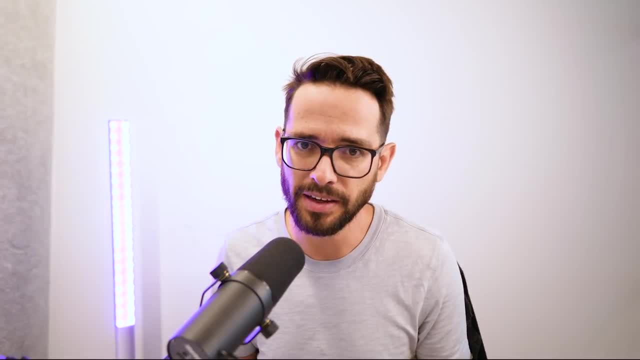 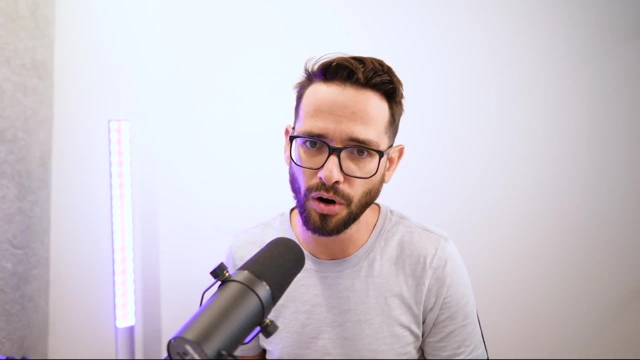 website is developed, developing it correctly, meaning that they'll be able to use some of the features like voice activation and stuff like that, And as designers who are basically managing the project and obviously designing the visuals, but also a lot of times. 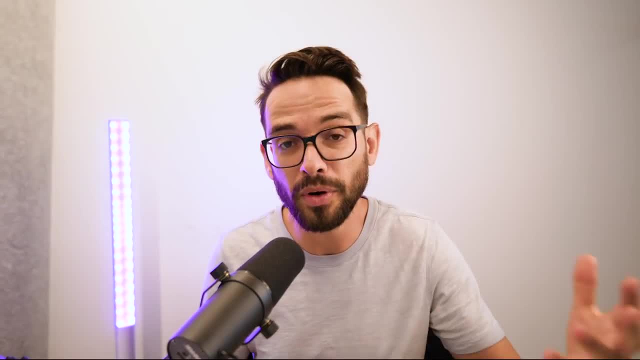 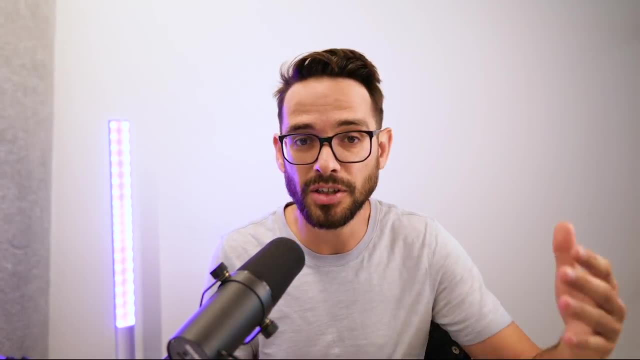 making sure that the development correlates to or we're actually managing the development. at least you know when I'm working and I'm actually building the website using Webflow, or you know managing developers. I have the responsibility of explaining to them what they. 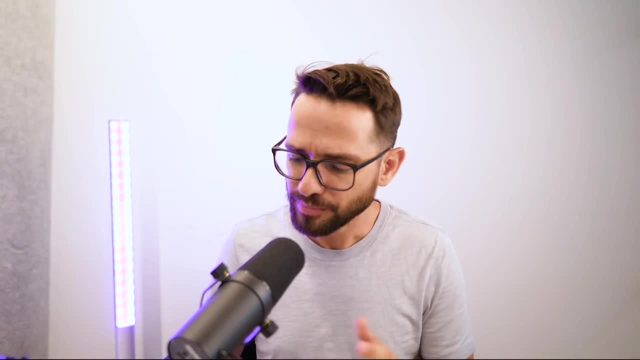 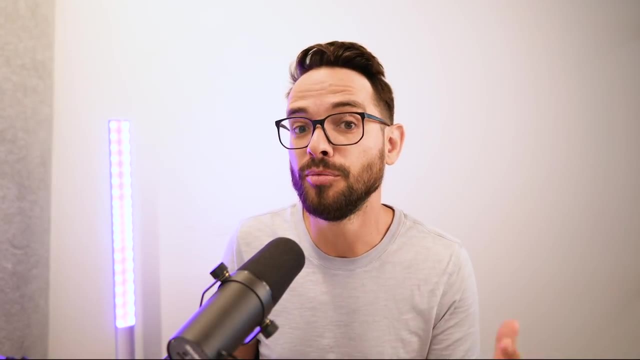 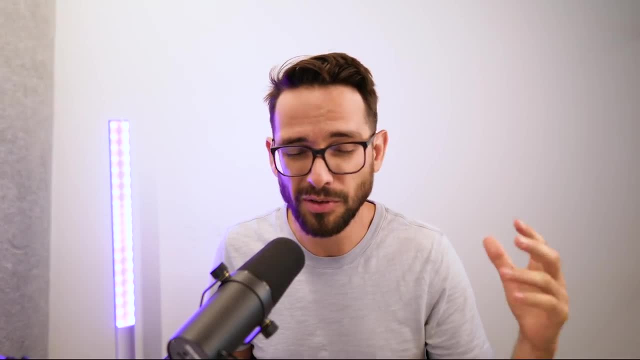 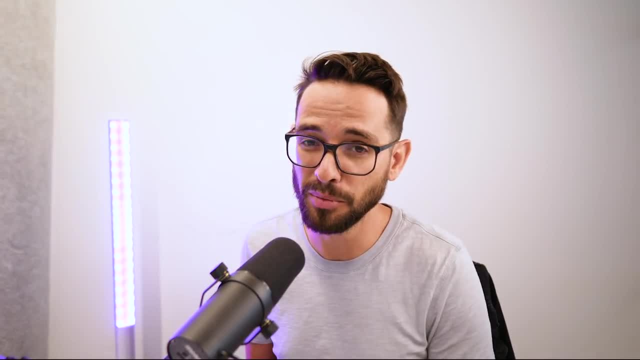 concepts in accessibility in a really fun Pablo Stanley way. So make sure to check the article. I'll cover some of the concept that he mentioned. I'll drill down on on some of them to make sure that you'll be able to implement it when you're designing for the web. So let's talk about kind. 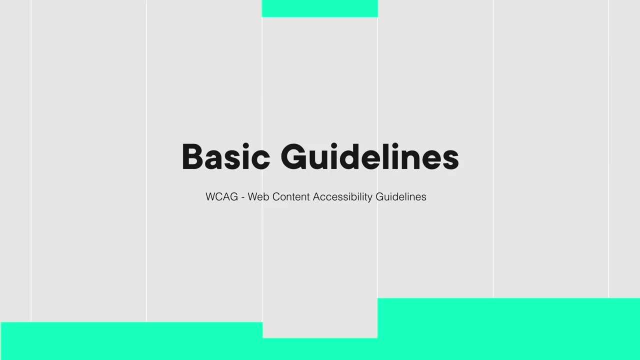 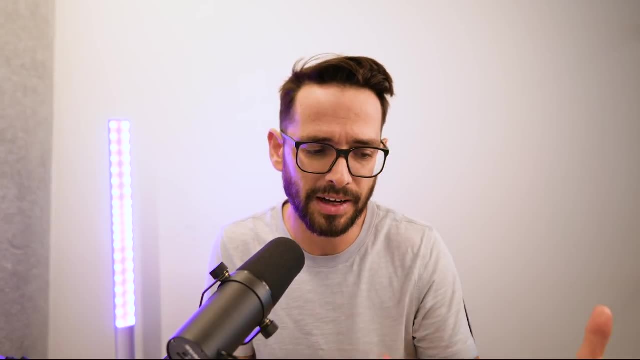 of like the key key concept- And, by the way, Pablo mentioned in this article that there is a Chrome extension that you can use to design for the web. So let's talk about kind of like the key key concept: install and that Chrome extension will show you if your website is already developed, what's what's. 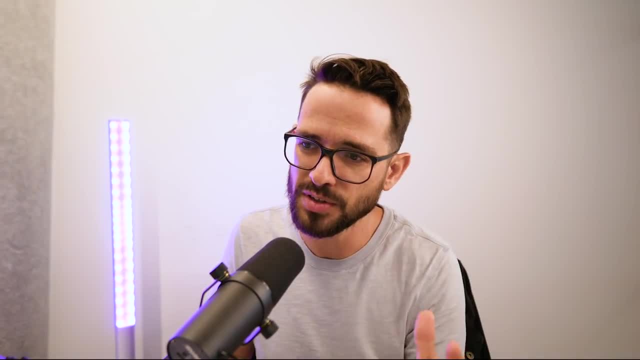 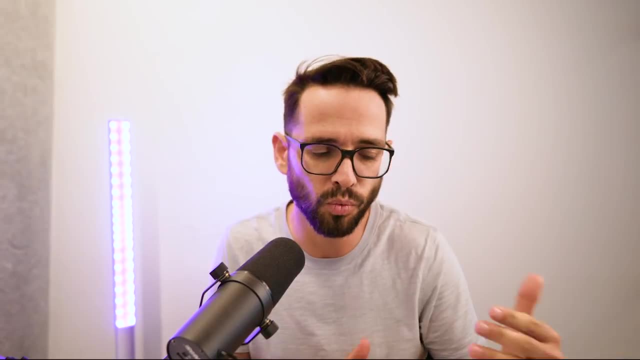 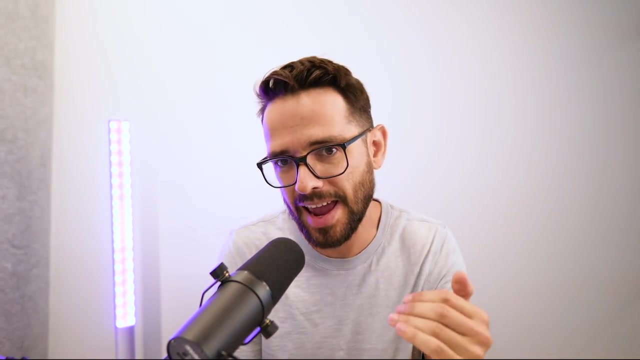 wrong and broken because there is what's called the WCAG, which is the Web Content Accessibility Guidelines. It's kind of a bunch of people who decide: what are they? what means that a website is accessible, what has to happen? And there's actually some rankings like a double A and triple. 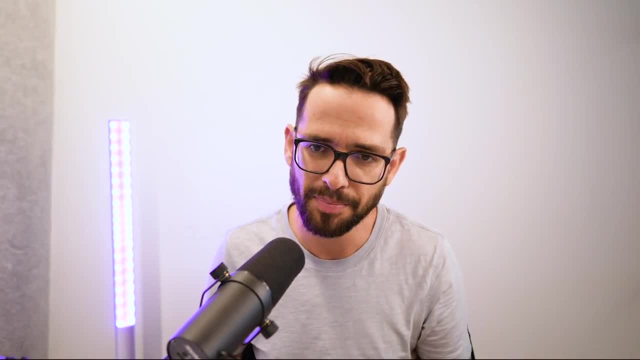 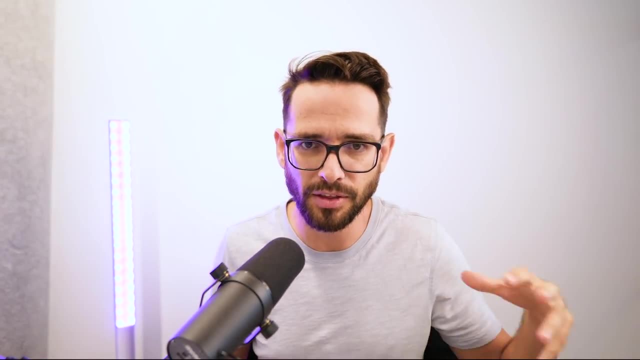 A, which means how good or how accessible your website is. So I'm not going to drill down to every tiny law here. I just want to cover the, the basic concept with you. But the, the Chrome extension that I've mentioned, does go in depth and tells you: 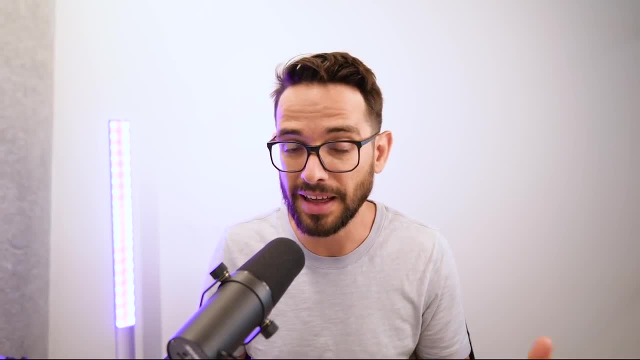 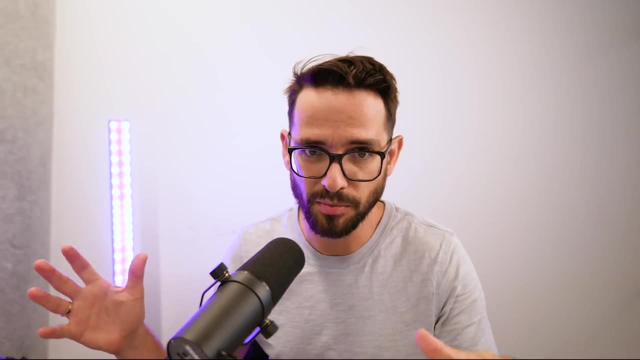 oh, this font is a little bit too small and stuff like that, So you might want to check out. it'll be in the description as well. Check it out and it'll help you. But let's get start with the main concept before you even have a website that's designed and developed. So the first concept is: 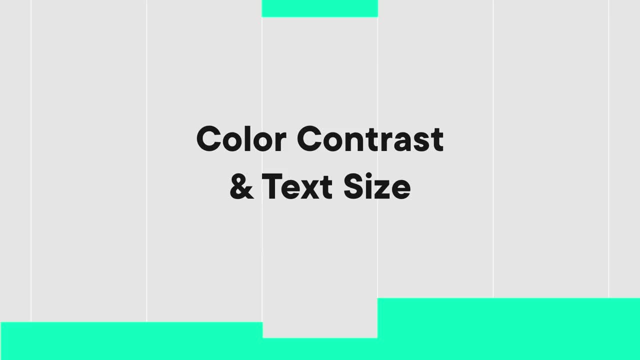 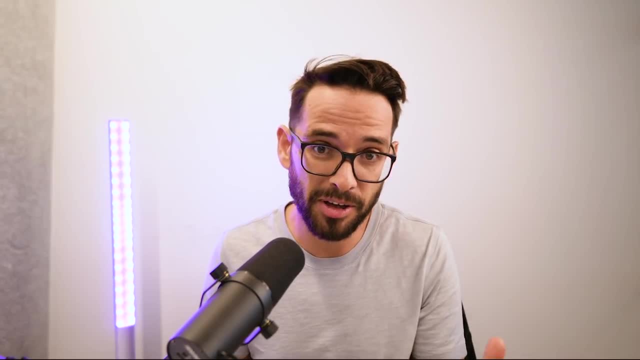 color contrast, And that's what I'm going to talk about in this video. So let's get started, And the idea here is that, as I said, some people- maybe old people or maybe people that have some visual impurities- can't see as good, And maybe you know we're designers. we usually work, maybe. 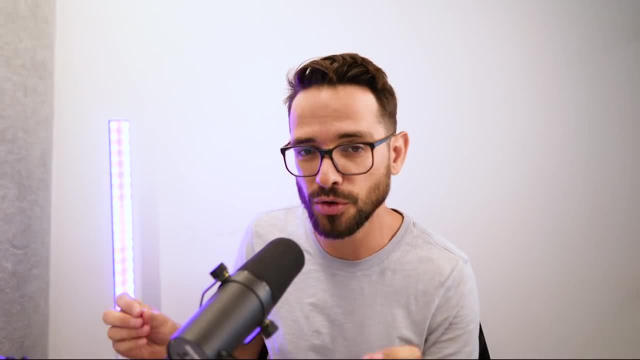 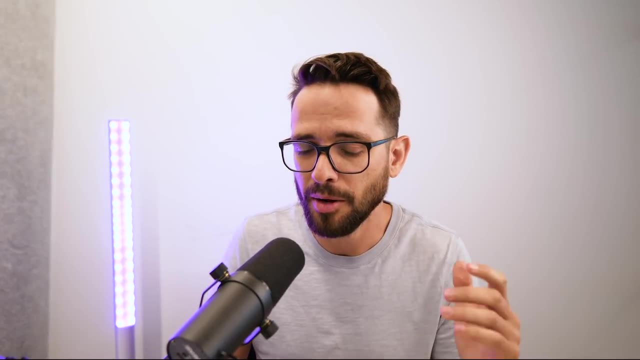 on a Mac or on a fancy, on a fancy display that shows color, really, really nice, And so we like to create hierarchies with, like, let's say, some kind of a shade of gray or something. But for people who can't see super, super well or have an amazing display like we have, that makes reading. 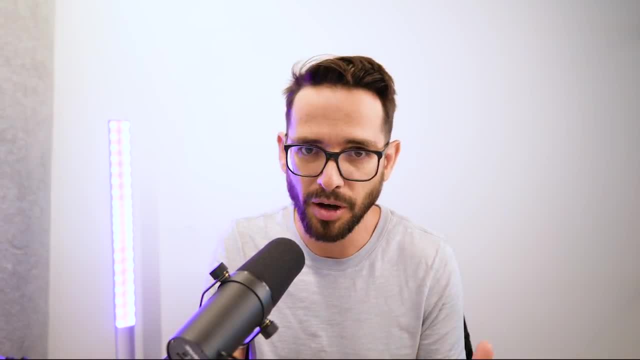 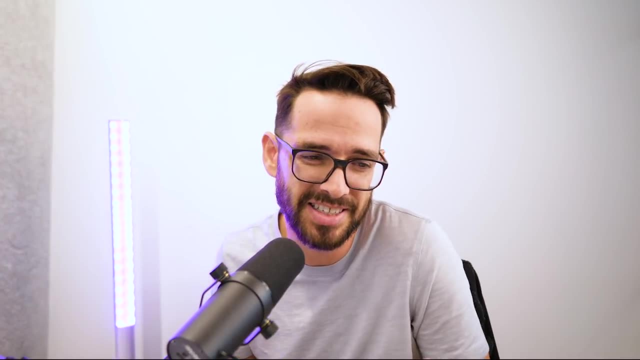 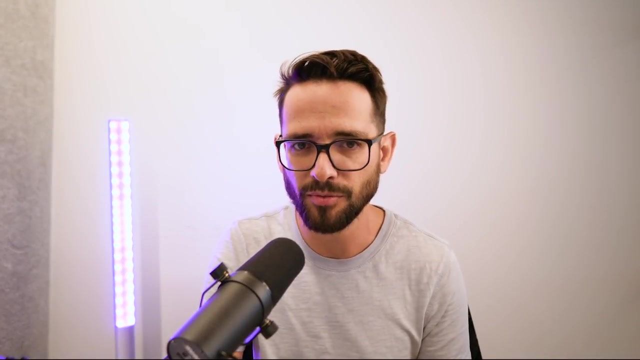 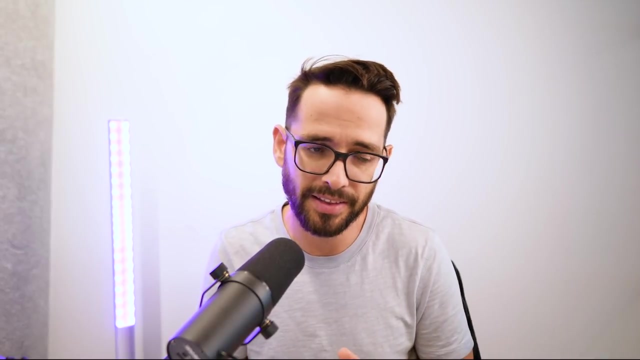 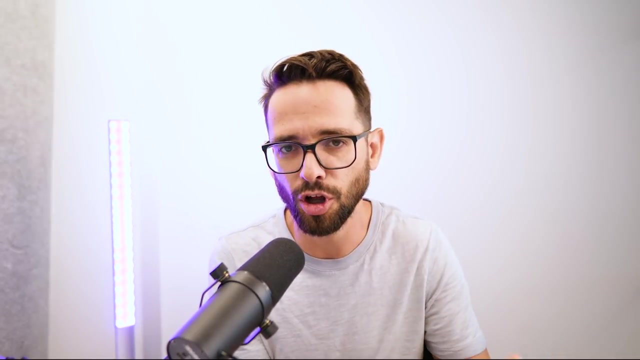 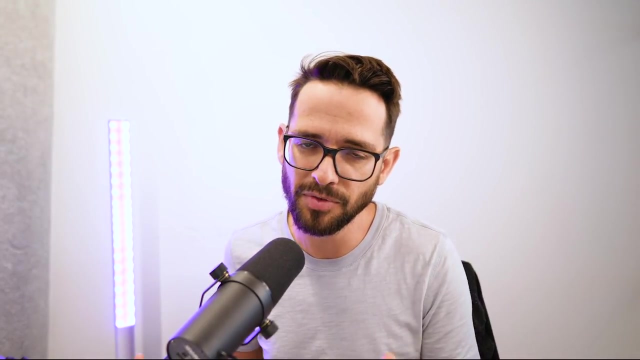 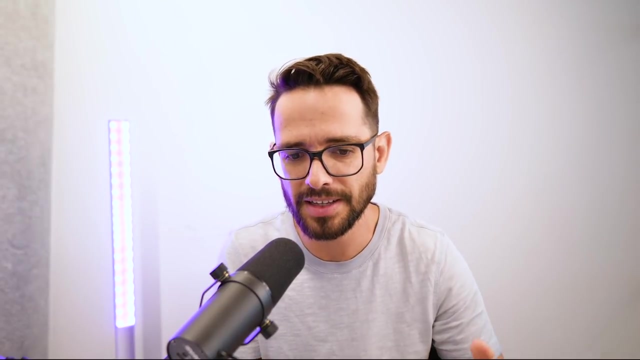 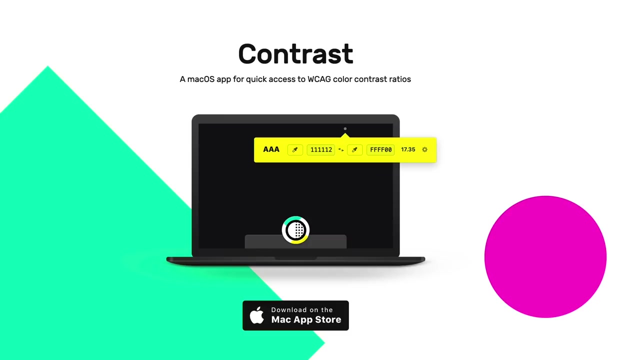 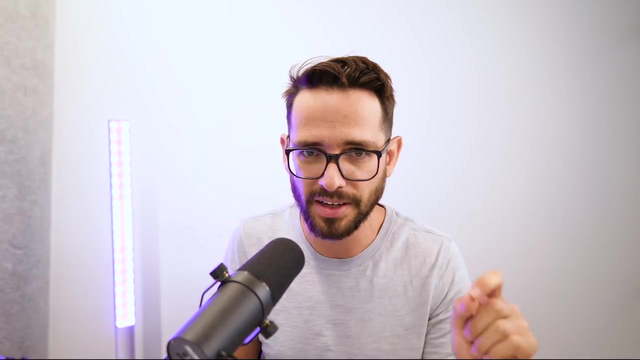 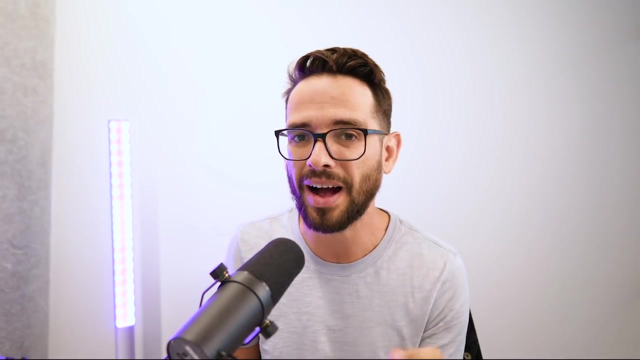 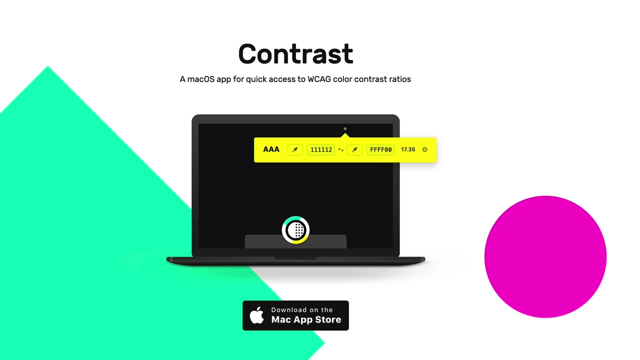 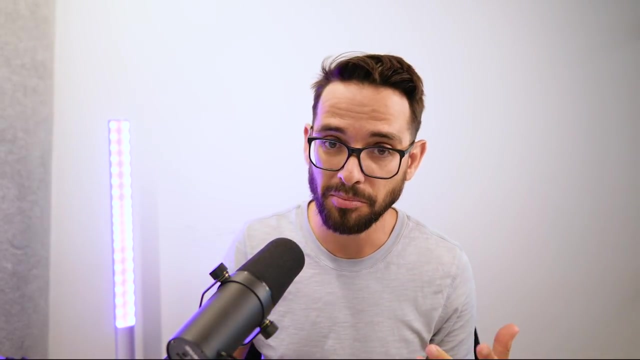 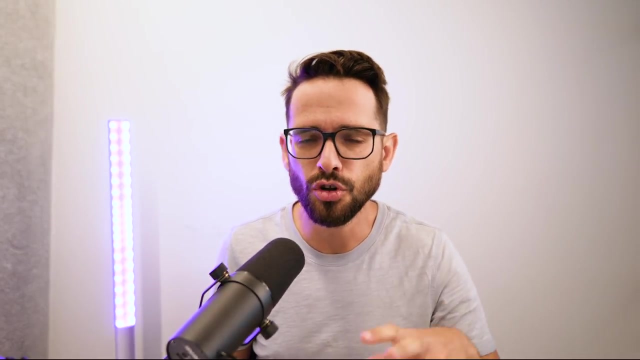 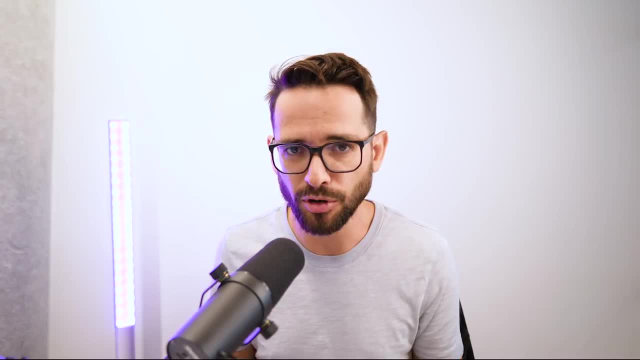 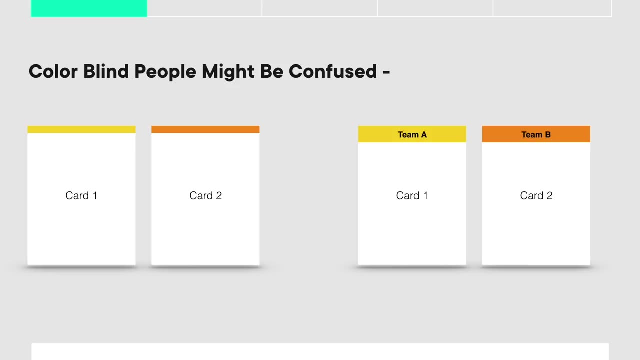 kind of difference differentiations, right, Because some people are colorblind and they might not see the difference. So let me give you an example. So let's say here, if you look at the right, we have two types of card and one of them is labeled with a yellow and one of them is labeled: 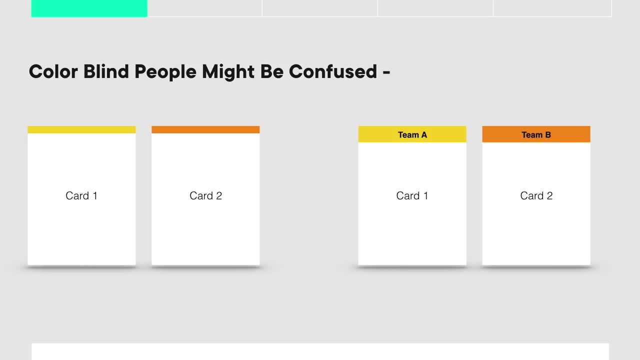 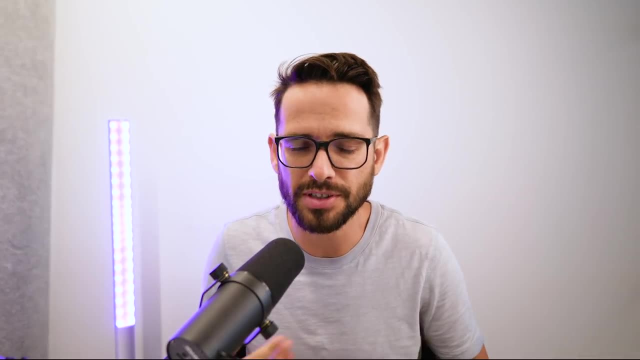 with an orange, but somebody that has colorblindness might not actually see that they are different. And if you're imagine that you're designing some kind of maybe a task management or something like that and you want to show a status of a project, if you're going to be only relying on 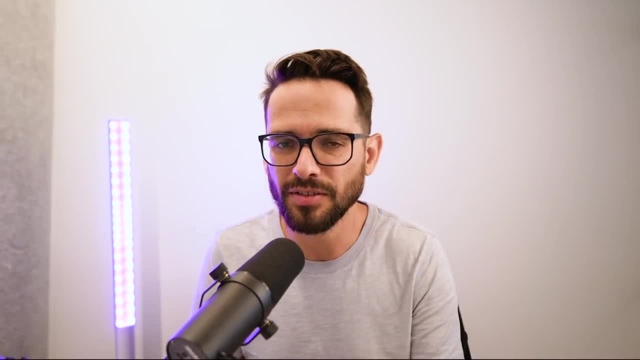 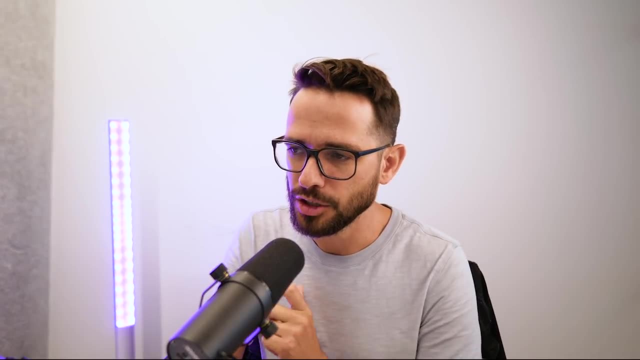 color, then somebody that's looking at it might not even see that there's a difference or urgency or something like that. So make sure that when you're designing, you add something else to this besides color. For example, if you look at the example on the right, I've added, for example: 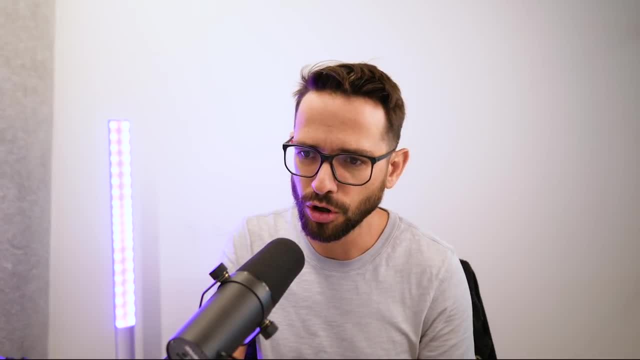 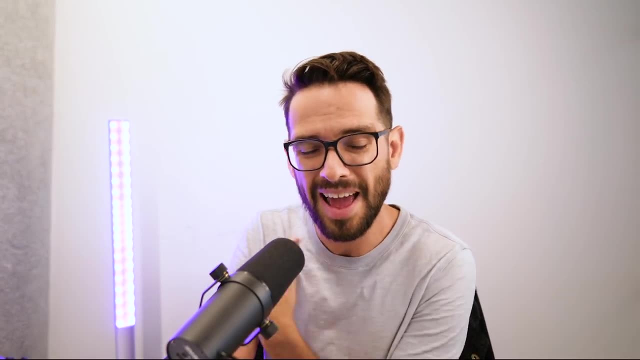 team A and team B. So it's not only relying on color. Obviously, for those of us who can see well, we're going to be able to make decisions or understand very quickly because of the help of color. but color is not the only way that's going to help us. 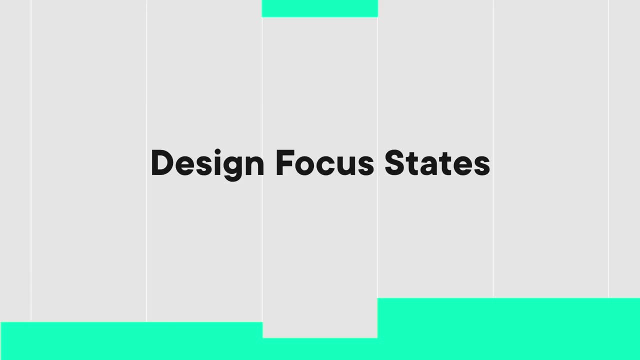 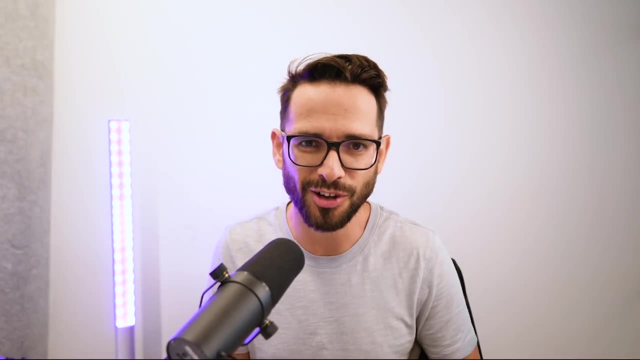 understand what's going on here, All right. So one more thing that you should care about is focus states. So we, as designers, obviously we like to focus a lot on hover states, and you know what happens when people move and hover with the mouse over something. 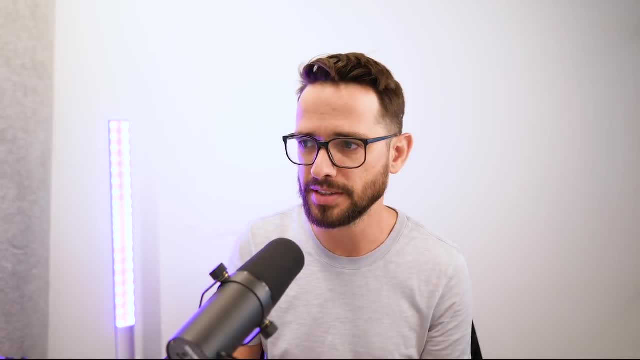 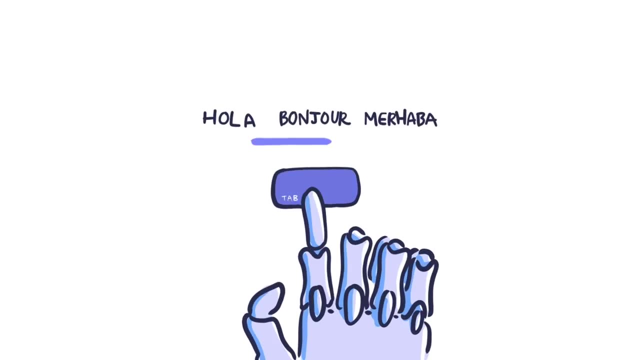 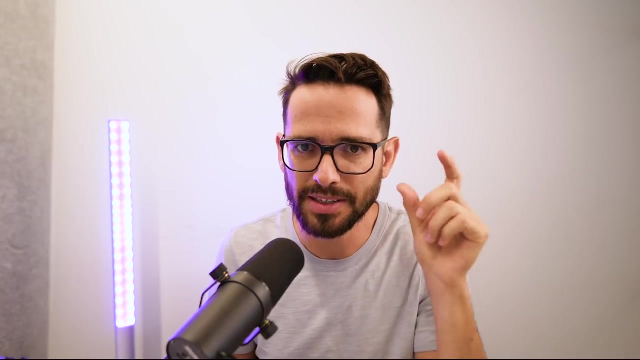 create fancy interactions But we a lot of times forget about the focus states. So focus states basically is for people who use the keyboard to navigate websites and stuff like that, So they might click the tab and then they kind of the selected link is going to be somehow. 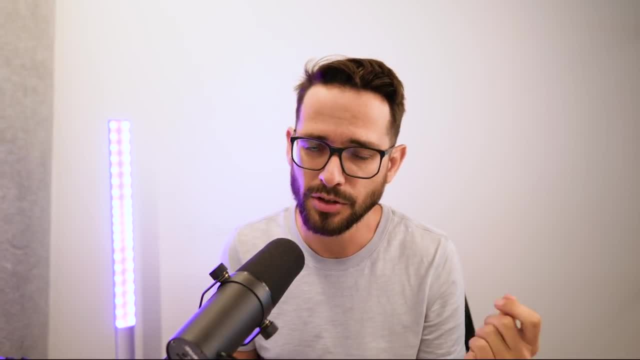 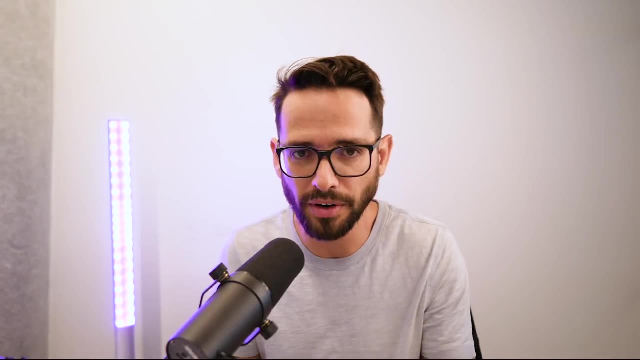 selected right And we need to show how that looks like. So this state is called focus state, and a lot of designers don't even bother designing it or telling the developers that they should implement this, because, again, this is not something that's visible. 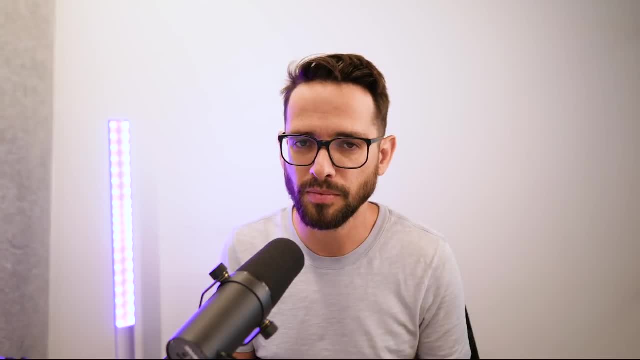 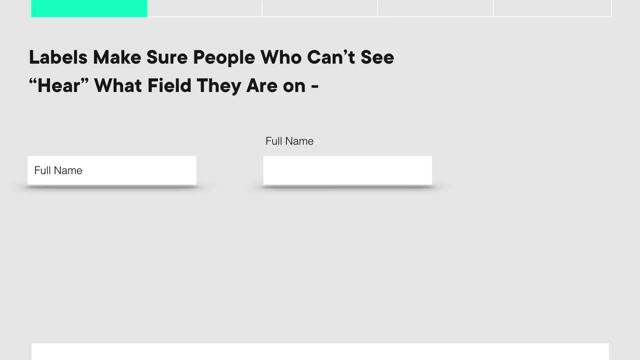 or used by them, And so they forget about it. So make sure that you also design for the focus state for people who are using tab to select and then navigate through the websites. All right, One more thing is labels. So these days, a lot of kind of trendy or this kind of design that you 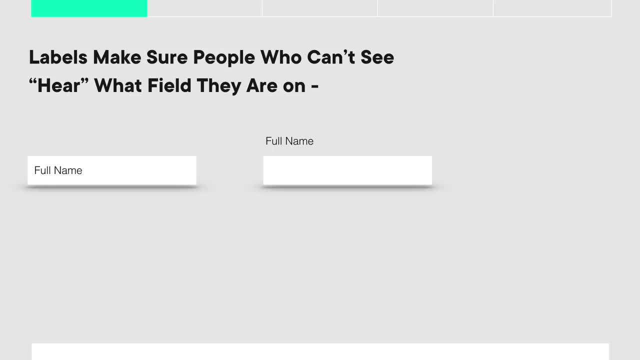 might see on Dribbble or stuff like that, when people are designing forms. it's very kind of minimalistic right, So it's like the example on the left. they're not even labeled for the form, And by label is what you see on the right when you have kind of a text that. 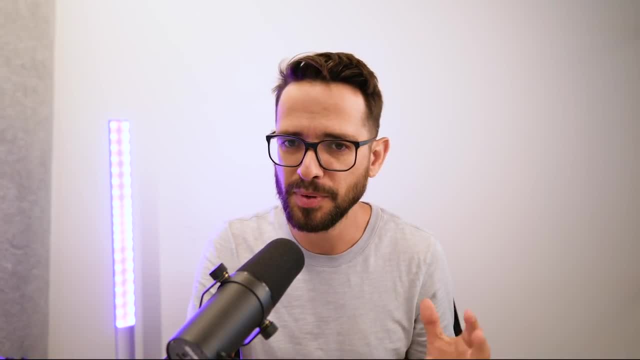 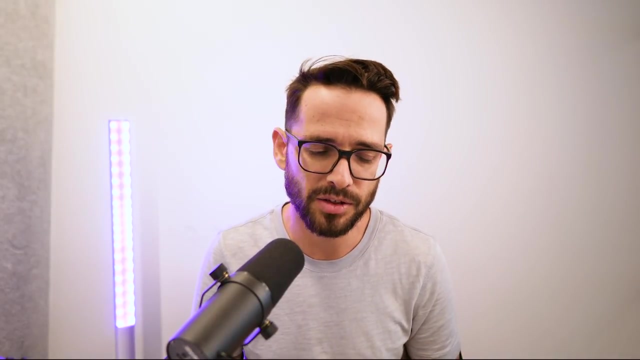 is above the form field. So a lot of times people would just use what's called the placeholder text inside the label to specify what this label is for. So again, like the example on the left, you can see that the full name is actually not a label. It's what's called a placeholder text. 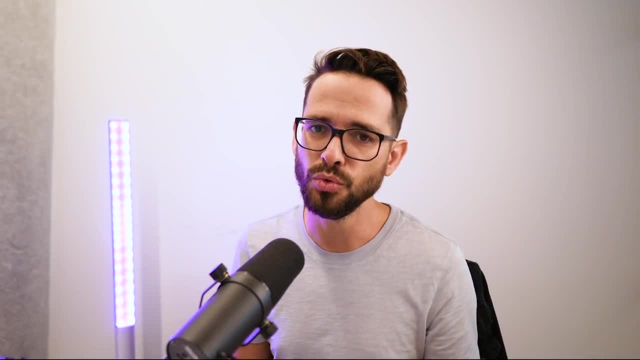 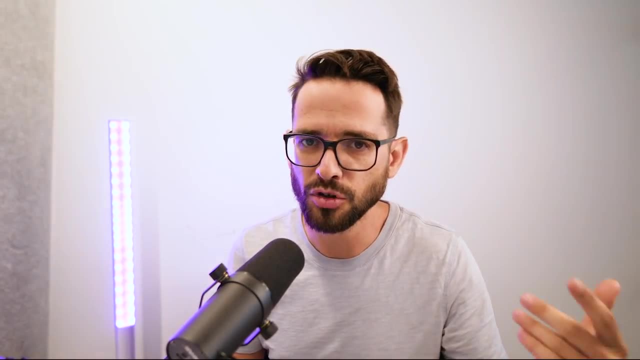 Now, the problem with this is, as I've mentioned, some people use tools that read the text, but they don't read the text, So they don't read the text, So they don't read the websites to them, And when there is no label, they're not going to be able to know what. 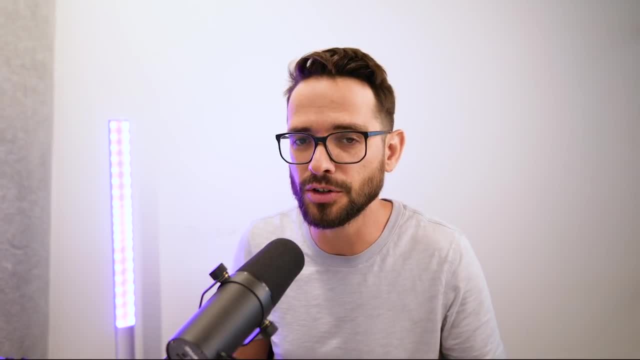 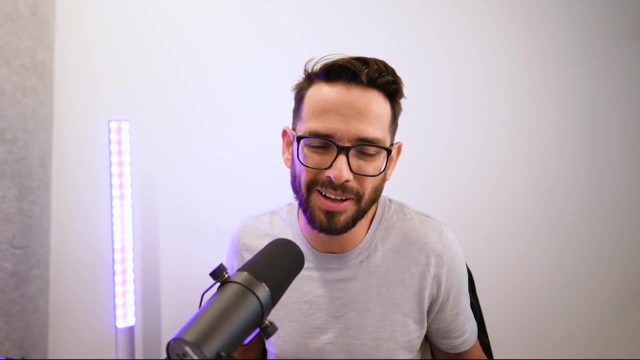 this form field is just because the website readers actually read the labels of the form. So you have to have kind of a label for the form. just build it this way, Otherwise they won't be able to know what this form is for and won't be able to fill it out. 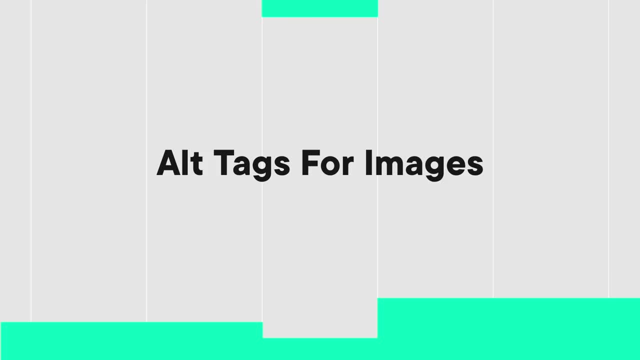 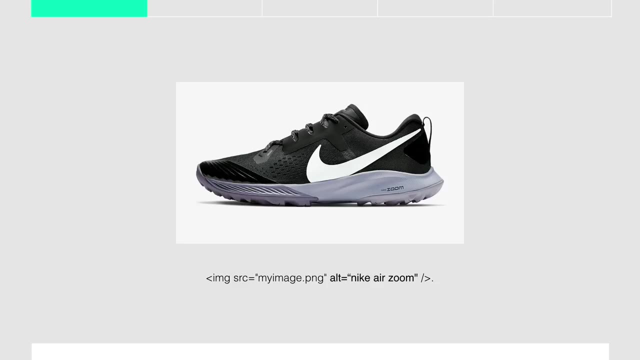 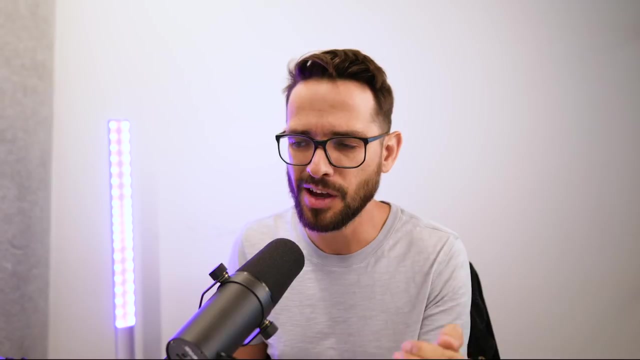 All right, Next thing is alt tabs. Now, alt tabs is basically when you design some kind of a website with a code that says, for example, show this image. An alt tag is a piece of the code, some letters inside the code, that actually explains what this image is. So, again, as you can see in 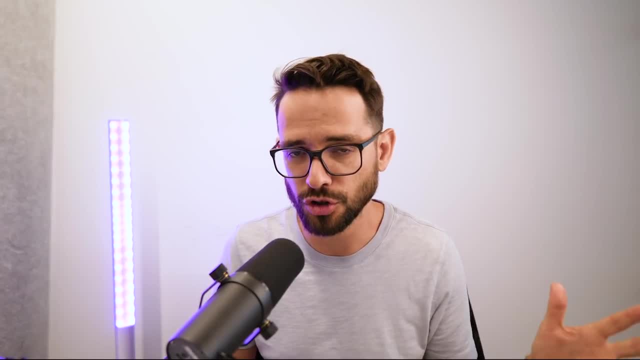 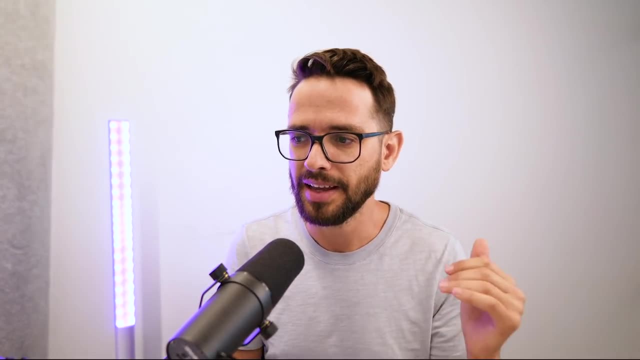 this example. here we have alt. By the way, alt stands for alternative, So if you can't see it and a machine is going to read the website to you for this image, it's going to say Nike Air Zoom, so that you can understand. if you can't see what's on the website, what's in there. 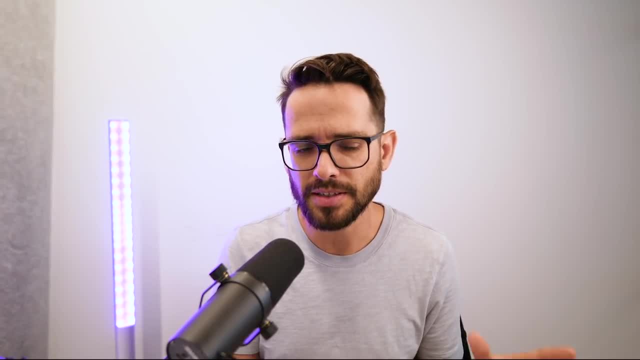 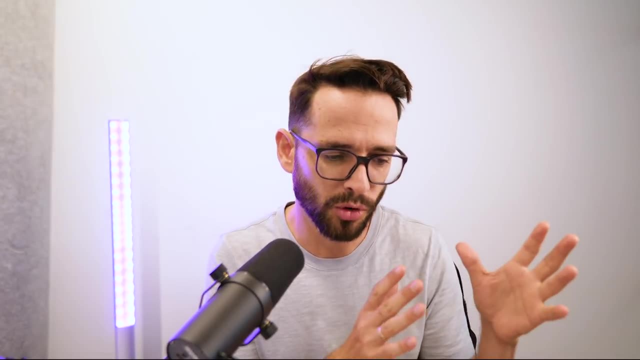 Now again, this is part of the development process. When you design, when you're working in Sketch, alt tags is meaningless, But when you're making the transition from your Sketch files into Webflow or working with a developer or whatever the way that you're building your website, 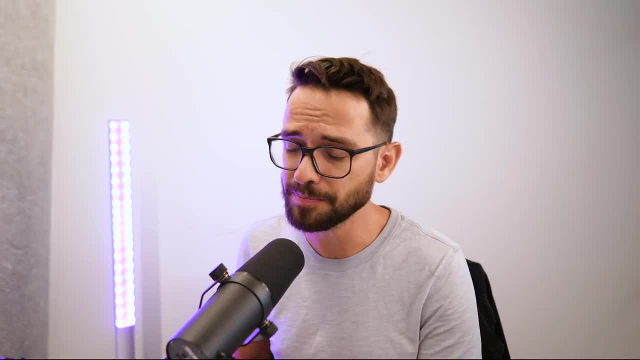 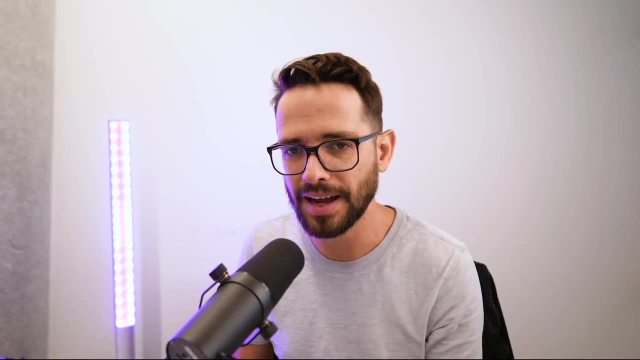 you must have a system for putting these alt tags in place. Also, if you're going to hand over the website to your client, you have to educate them about alt tags and how, whenever they, let's say, put in a new blog post. 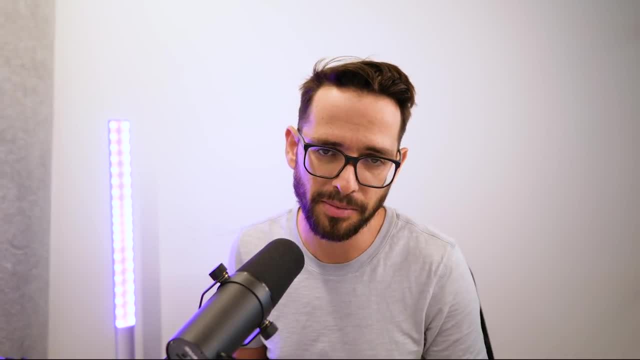 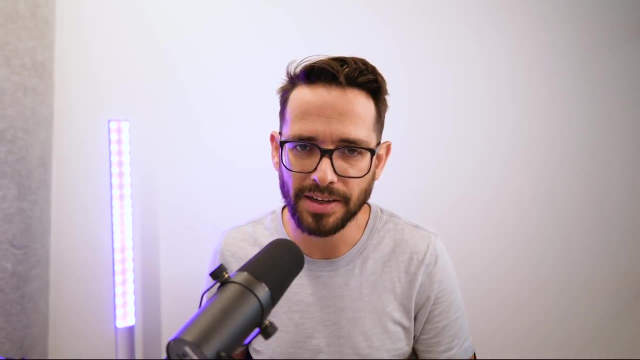 or update content in their website, they should be using alt tags to make sure that their website is accessible right. So this kind of leads into how to make sure that the website is developed correctly, And it has to do with things like how to set up the correct markup. 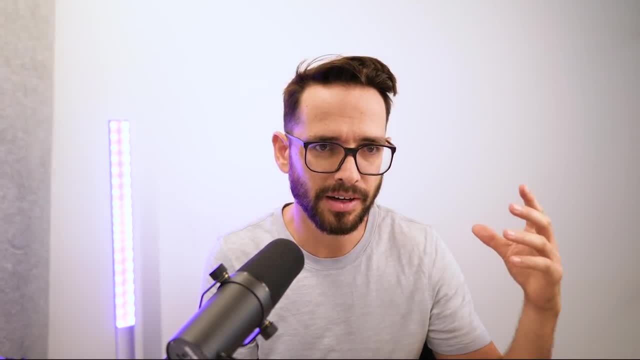 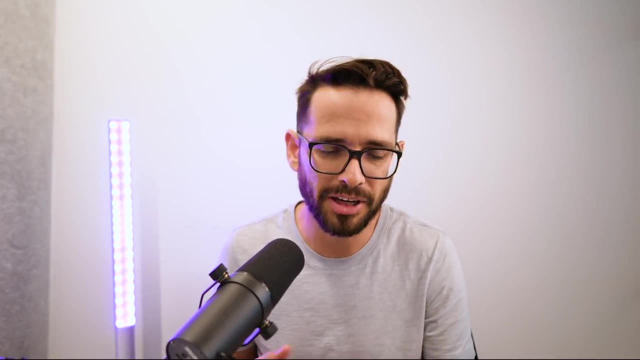 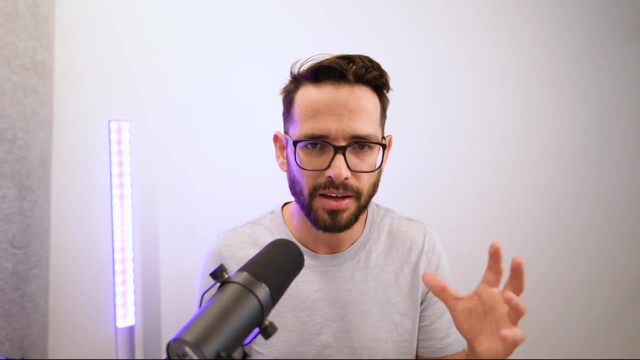 which means, let's say that the code is written correctly so that they would know what an article is, what a navigation is, what a footer is and how. to make sure that you know the website will be navigatable with keyboard And this gets a little bit technical. but again, it's not yours If 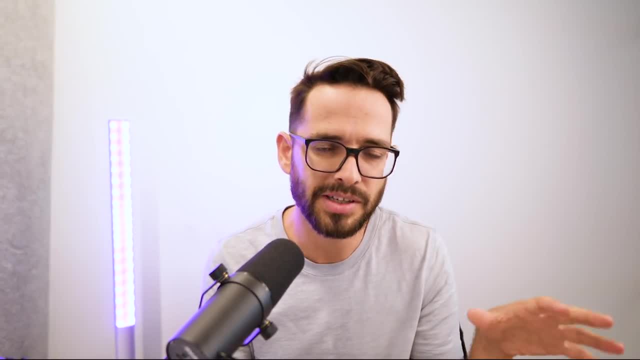 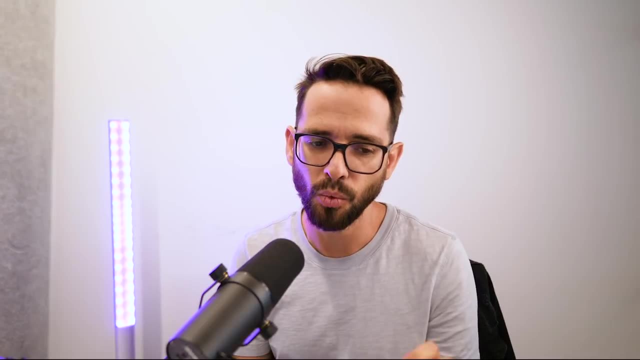 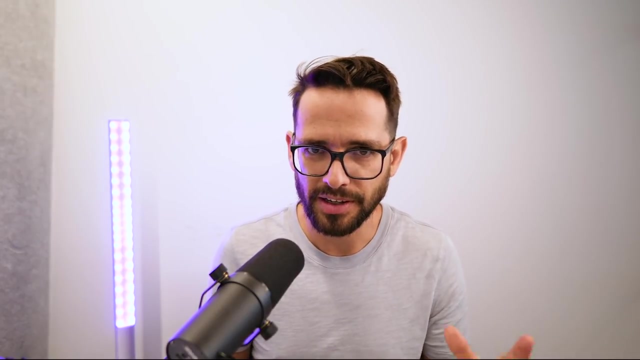 you're a designer and you're not developing yourself the website. obviously it's not your responsibility, but you have to educate, or you have to make sure that the developer that you're working with will do a good job by developing the website correctly. Now, as I've mentioned in the 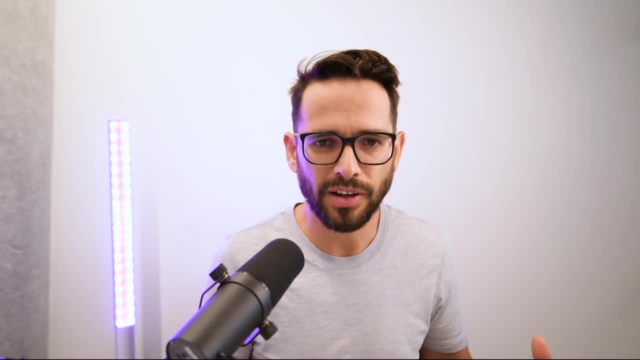 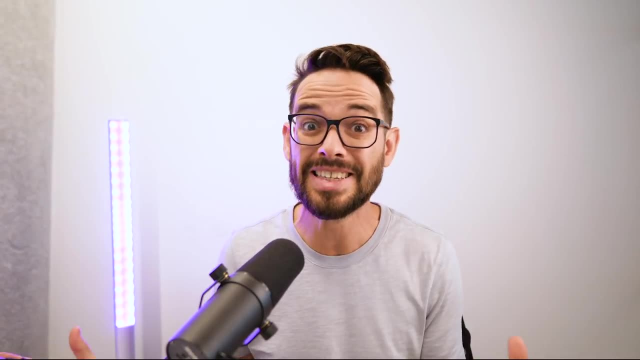 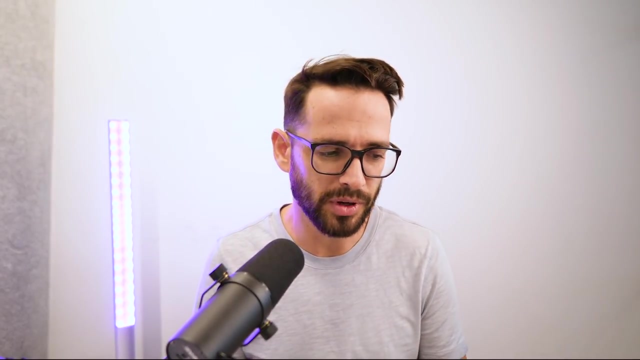 beginning of the video. now it's kind of like a little bit of scary in terms of lawsuit. is my website, you know, lawsuit safe And some clients are afraid of that? And because you know we are at the end of the day, we're designers, The law and if you're trying to read 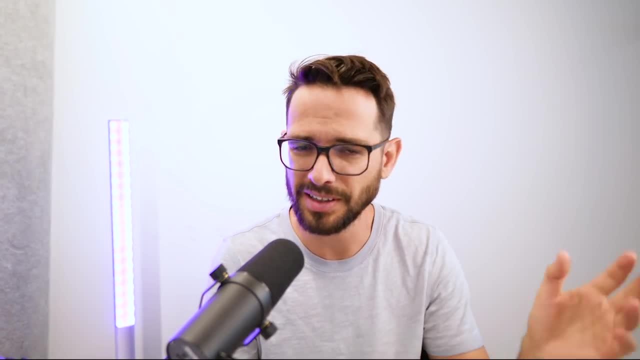 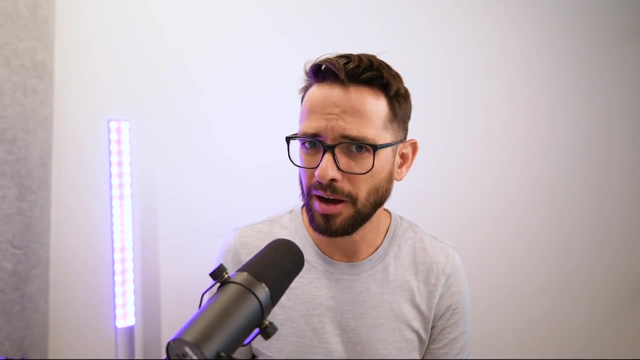 everything that's in the you know web content accessibility guideline. you might not understand everything. You might not be able to implement everything. So if your clients care about not being sued for you know accessibility issues, you want to make sure a hundred percent that. 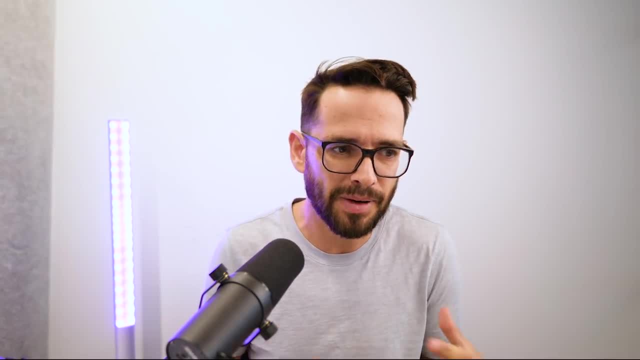 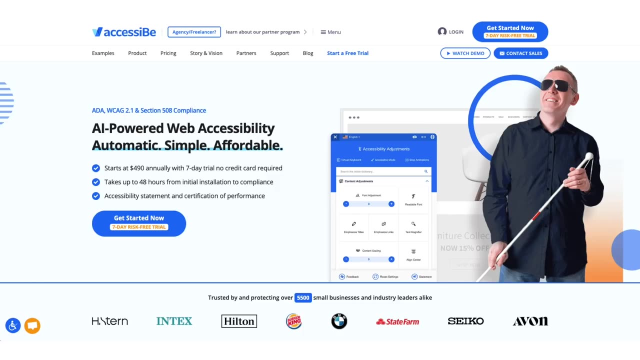 you know that you're safe. So in that case, I personally don't know everything that there is to know, And but there is a solution. So this is a company. AccessiBe is a company. Actually, I know these guys are based here in Israel and I've met them a few times and they've built. 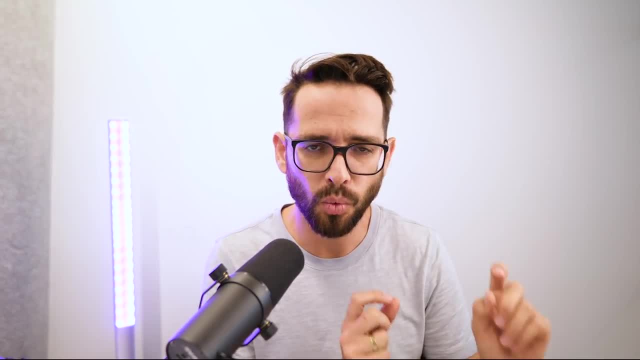 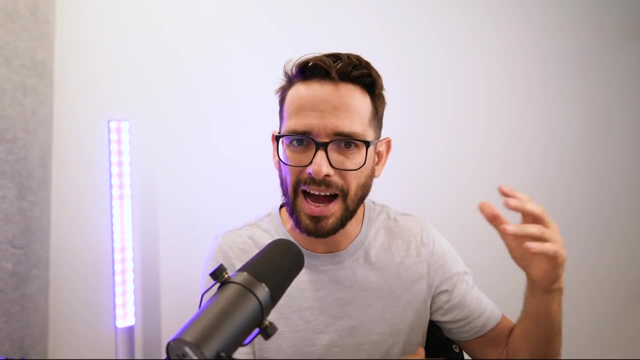 basically a product which, by just entering one line of code into your website, it takes care of basically two things. First of all, it kind of uses AI to put in all the out tags and change the markup to make sure that the development is developed according to the 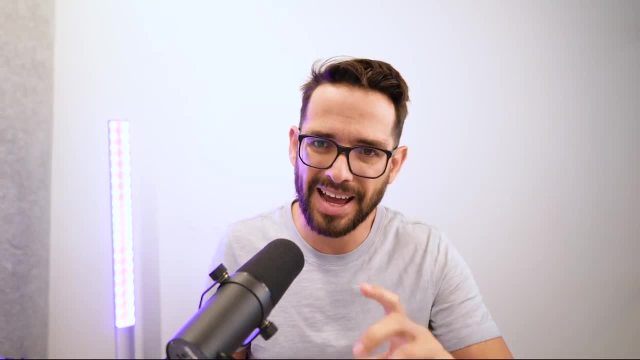 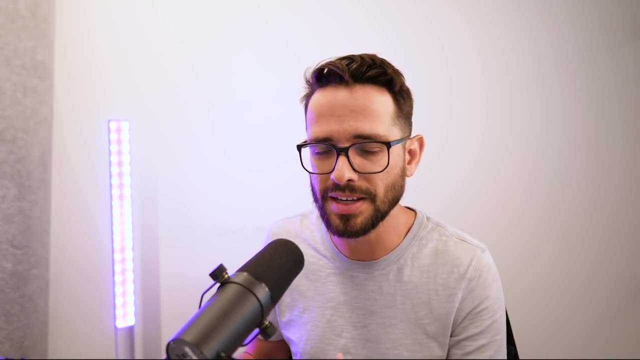 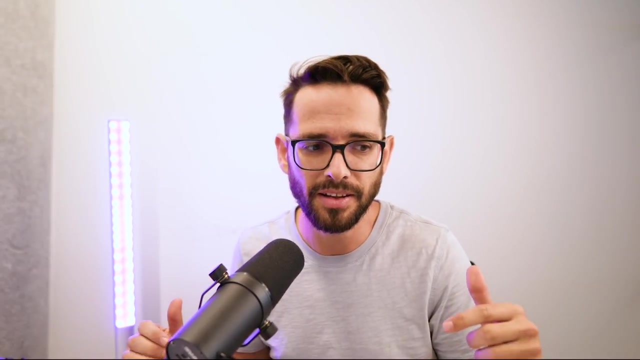 standard. That's one thing, And then on the visual side it kind of adds a little. if you want a little pop-up that can give you this kind of options to increase text size, contrast and stuff like that, So you don't have to. in some, in some countries, for example in Israel, it is legally. 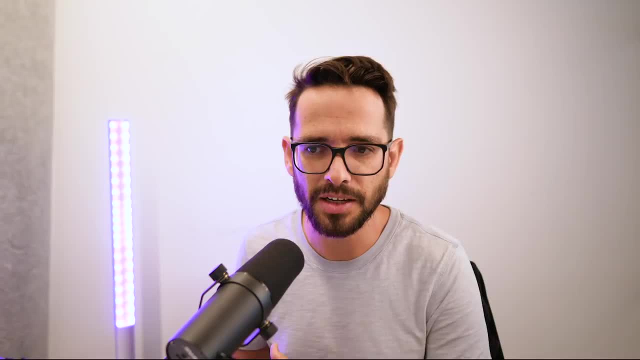 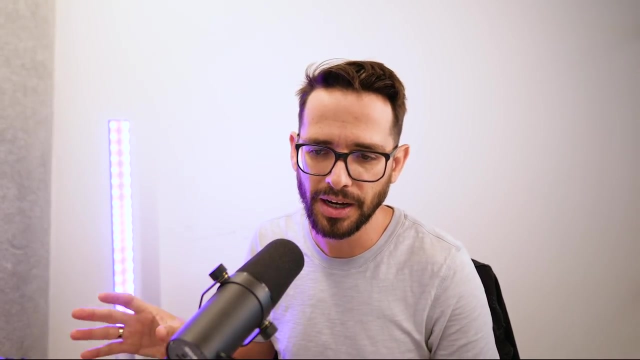 binding actually to put these kinds of pop-ups in every website to make sure that people who want to make the web, the font bigger or more contrast or see the black the website just black and white, can do that using some kind of a menu. So this tool actually helps you implement that inside the, you know, inside. 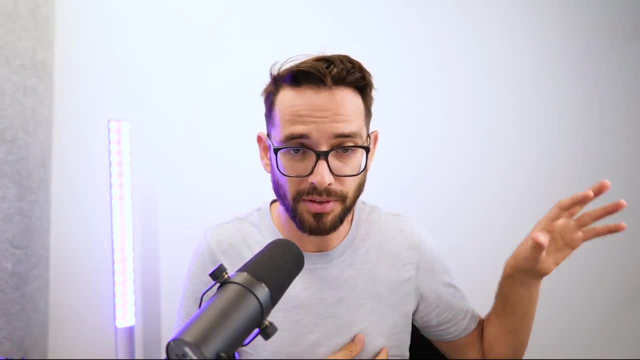 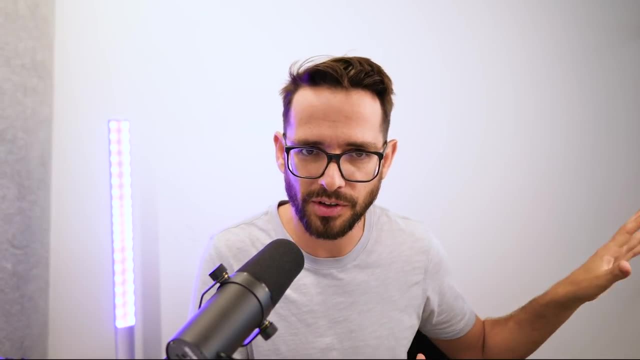 the tool. Now I have to be super, super honest that they are my friends. As I said, I never used actually their product in any of the website that I've built. This is not kind of a sponsored video. They did not ask me to do this, So I'm just like I've recommended. 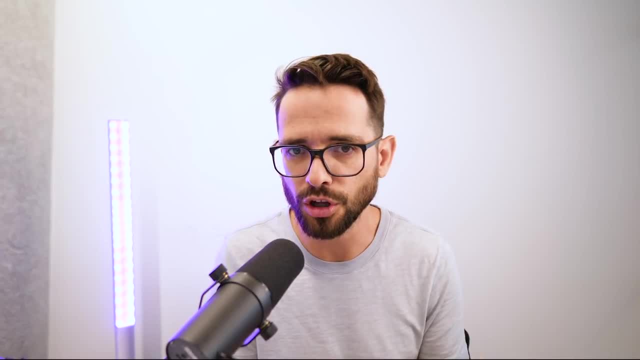 this product to a lot of my students in the Webflow Masterclass who were looking for a solution for making sure that their website are accessible, And I've heard great things about this. Again, I'd never used it personally, So I can only say that it looks great. It looks like a great solution. I've heard 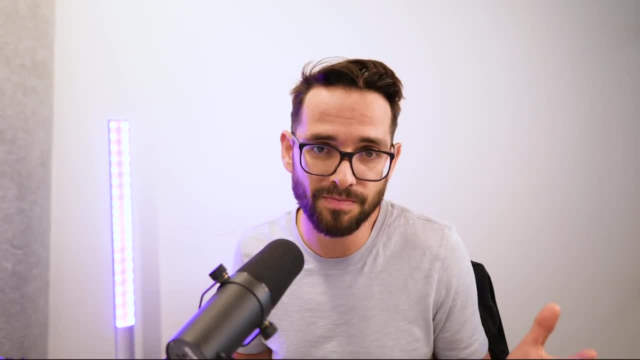 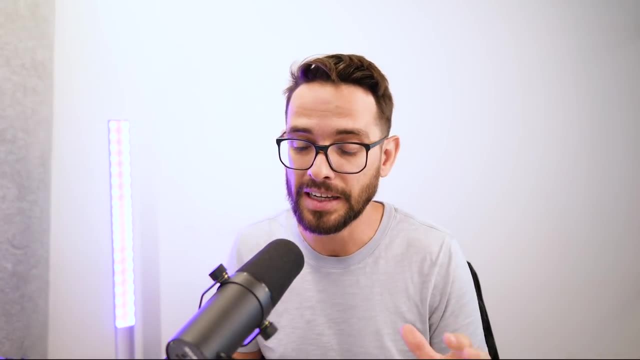 good things from my students, but you know, it's just. I'm just showing you that it's a solution if you're looking for it, and just just to make sure that you're legally covered. So I want to give you some final thoughts and be like super honest. 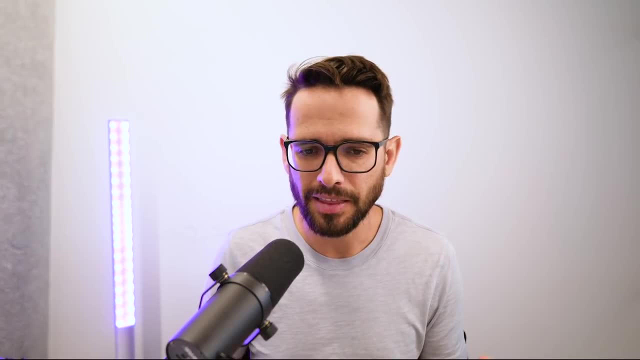 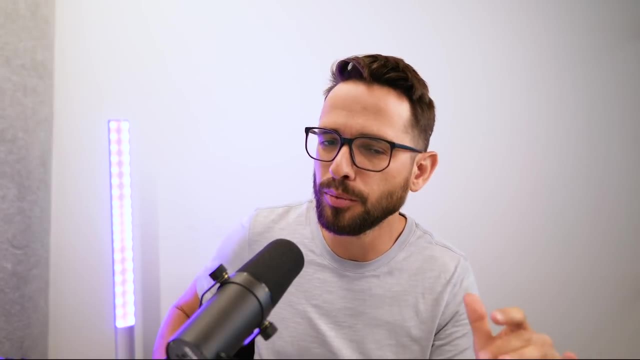 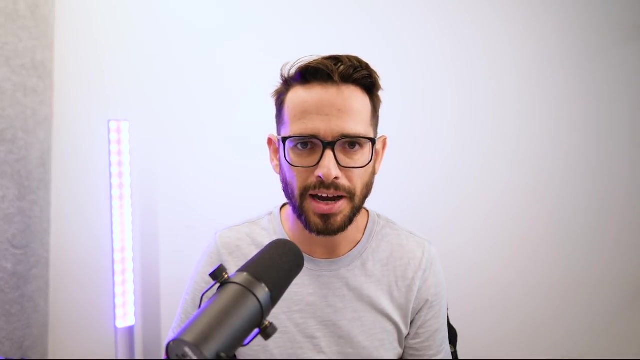 So I want to give you some final thoughts and be like super honest and open about this. Look, I have to admit that not every website that I've designed has been like 100 percent, fully like legal proof and and super accessible. This is something that's just. I feel like in the last two years have been gaining traction and shifting the mindset of designers. 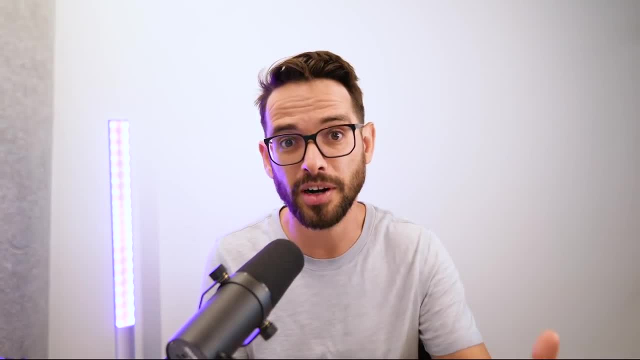 So I know I'm not like perfect- in that sense I'm trying to be better with every Web site that I'm designing- And also in terms of kind of like the, the, the, the, you know the process, and the kind of like the, the, you know the, the, the process, and the kind of like the, the, the, the, the, the process. 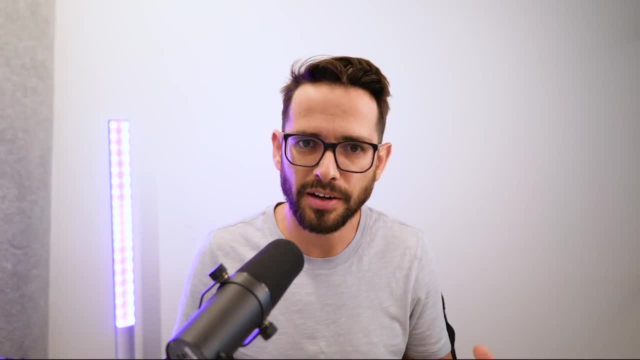 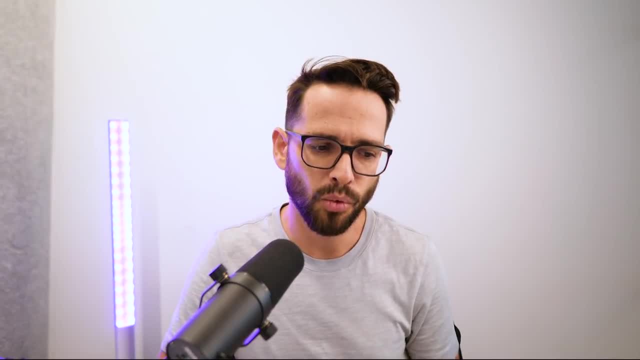 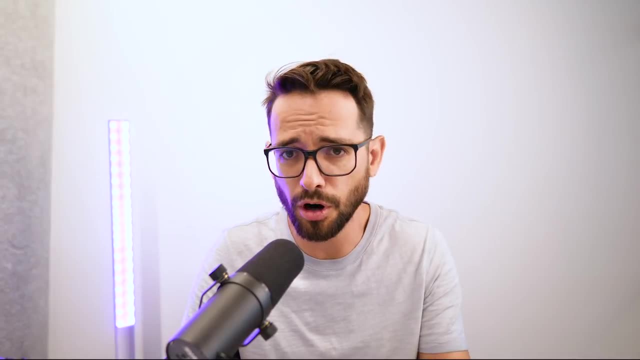 think it really depends on who your client is. i think that when you're kicking off a project with your client and you're getting to know them, you have to ask and you have to make sure, and it really depends on who their audience is and so forth. how important is accessibility for you as a client? 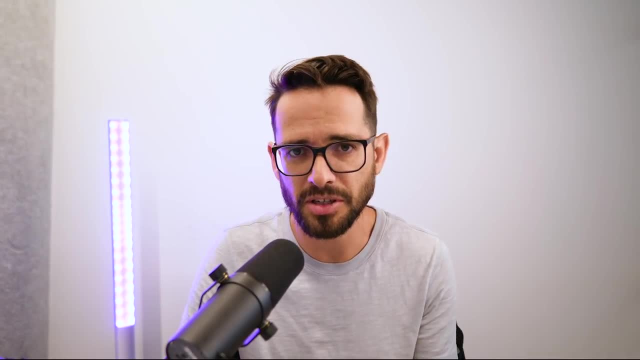 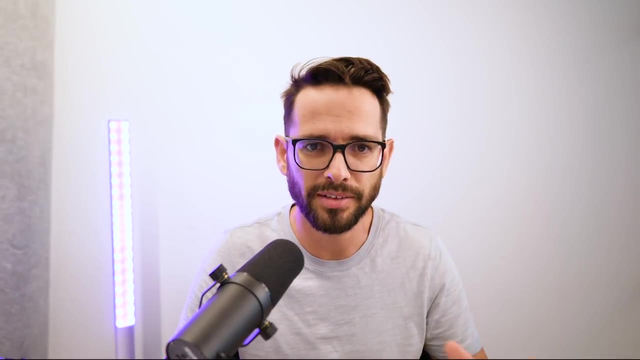 right, you, as, as a designer, you have to have the responsibility to educate them, to tell them what are the legal requirements. but again, you're not a lawyer, so you can't like fully. just like you have to tell them, put a privacy policy, but you don't really, you can't write the privacy policy. 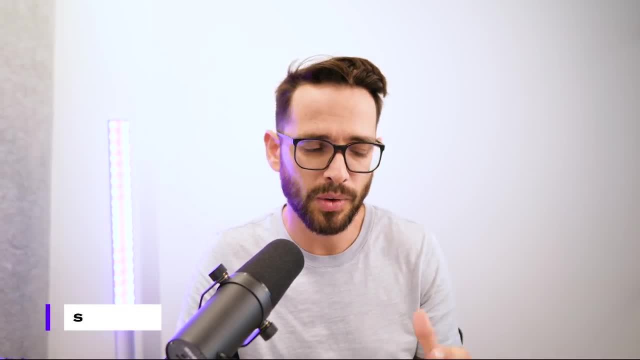 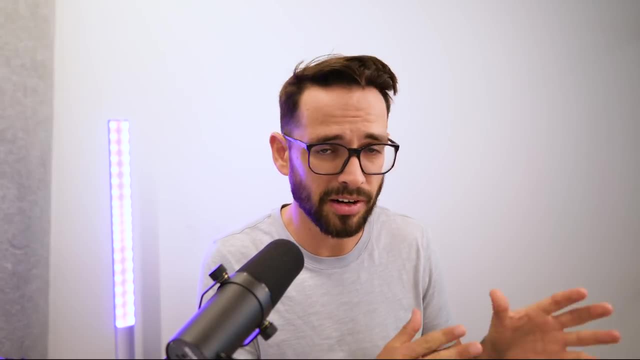 for them. i feel it's the same with you know, accessibility, you have to tell them it's a thing. you have to tell them what the options are. like you can say, from my end, i'm going to make sure that there's going to be enough contrast and everything, if you're taking care of development. 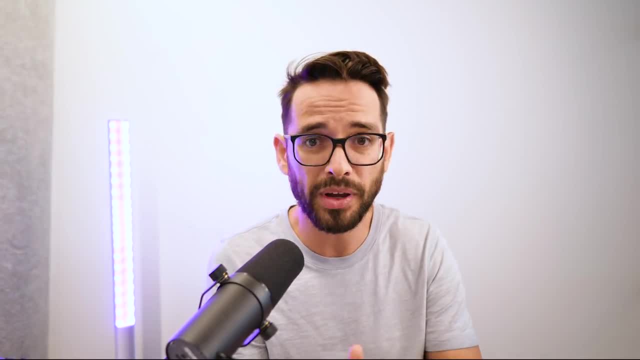 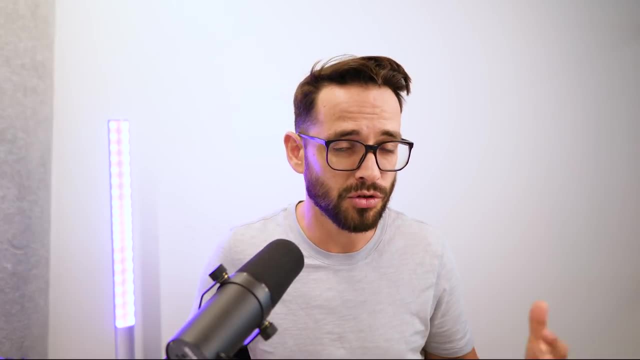 you're responsible for making sure that it's developed correctly. we can use this plugin or we cannot use this plugin. it's your. you know you're the client. you make the final decision. um, so just understand the context, uh, educate your clients and then make the right decisions, and i